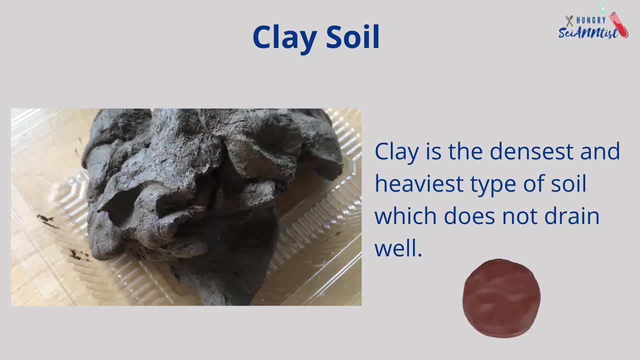 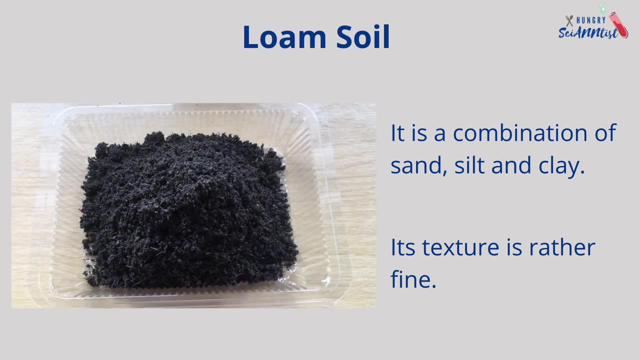 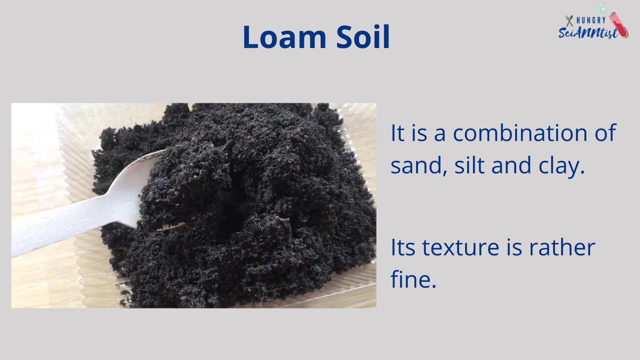 Clay is the densest and heaviest type of soil, which does not drain well- Loam soil: It is a combination of sand, silt and clay. Its texture is rather fine. It's black or brown because of a high amount of humus. 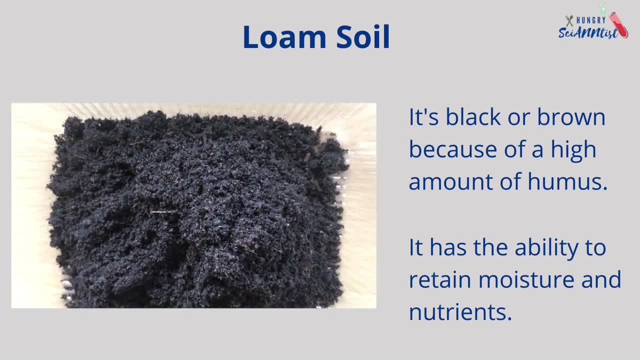 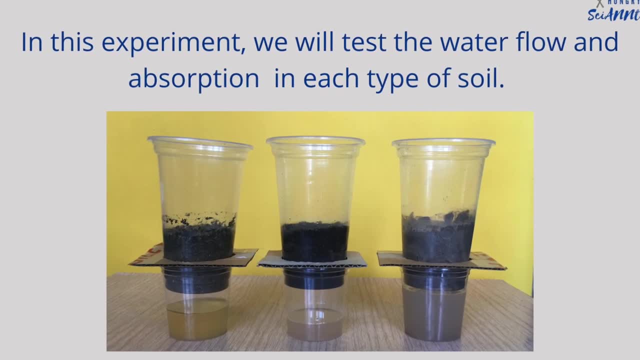 It has the ability to retain moisture and nutrients. The soil is high in nitrogen and potassium. It has a high concentration of nitrogen in its water content. In this experiment, we will test the water flow and absorption in each type of soil. I prepared three cups with holes. 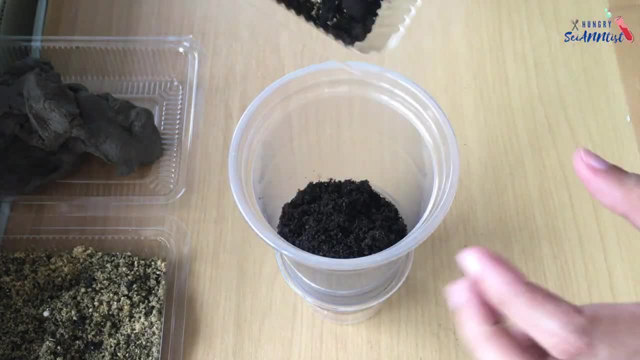 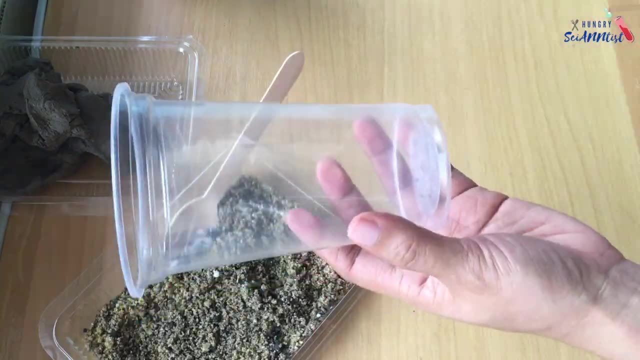 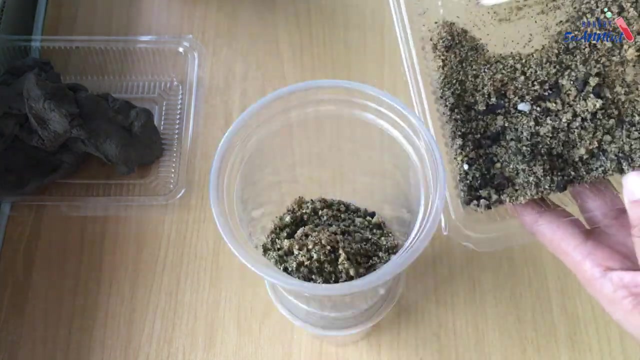 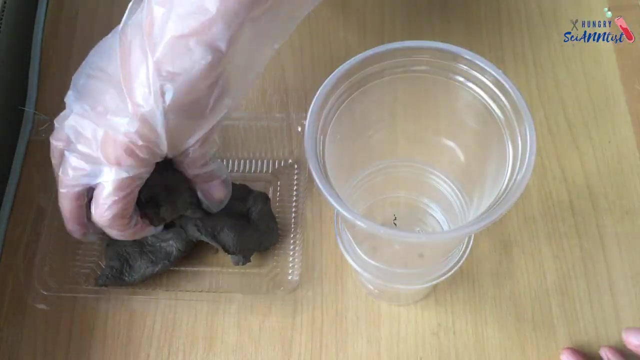 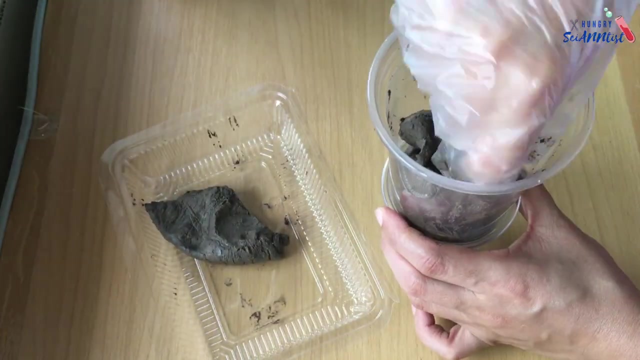 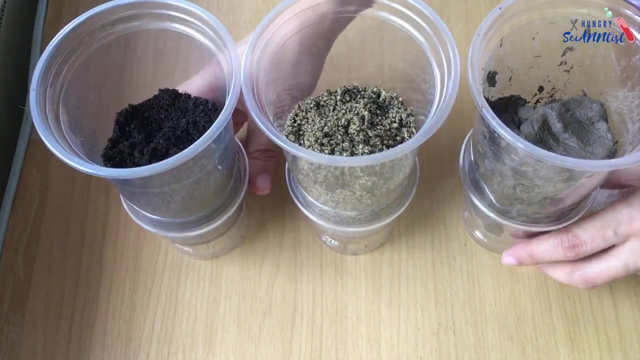 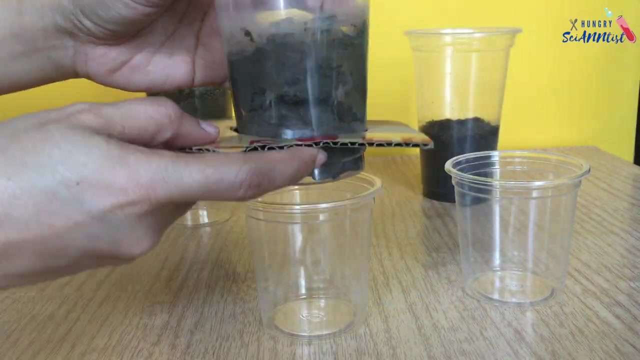 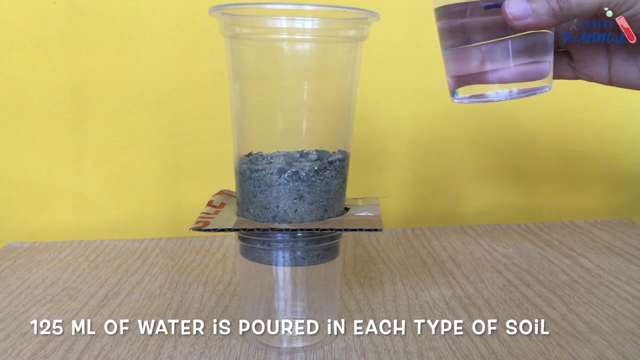 The temperature of the water has to be warm. Number of cups is different according to the soil. Water temperature is the same: It must be room temperature. The water level in the cup may vary depending on the type of soil. Thank you, The water is measured and the timer is set. 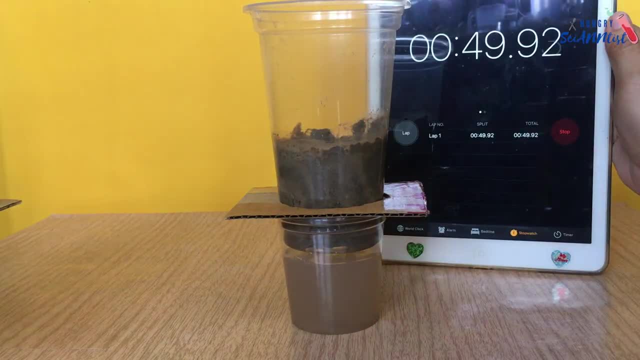 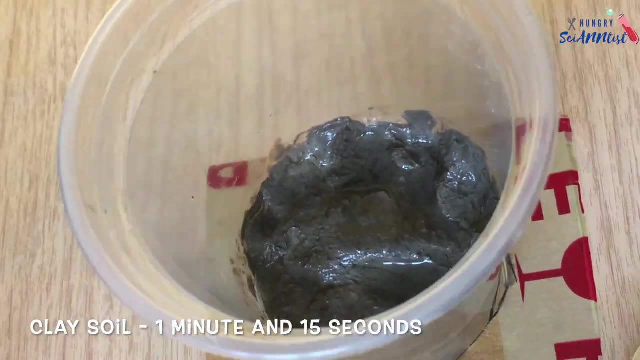 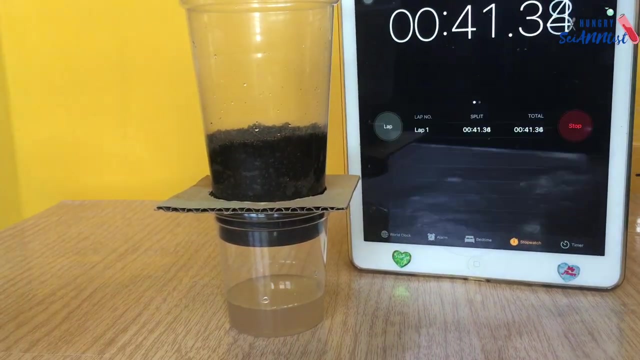 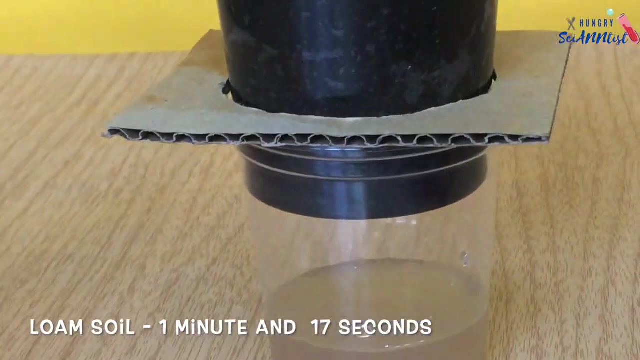 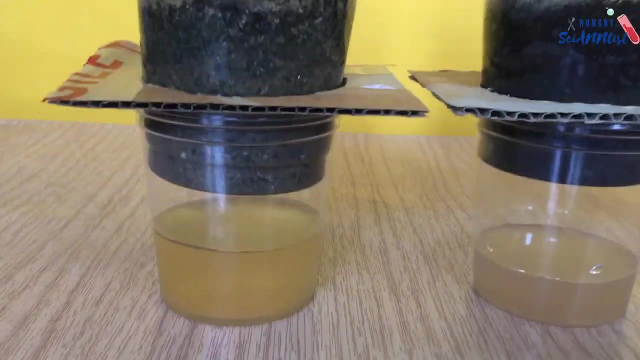 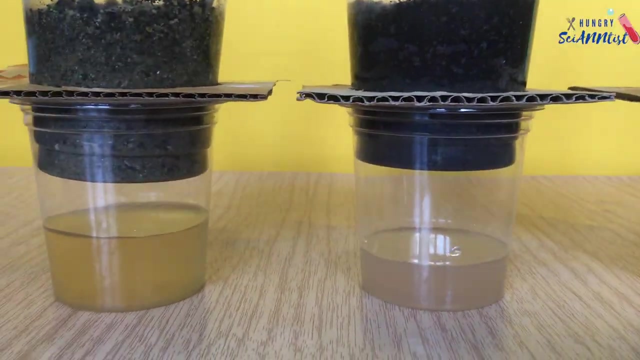 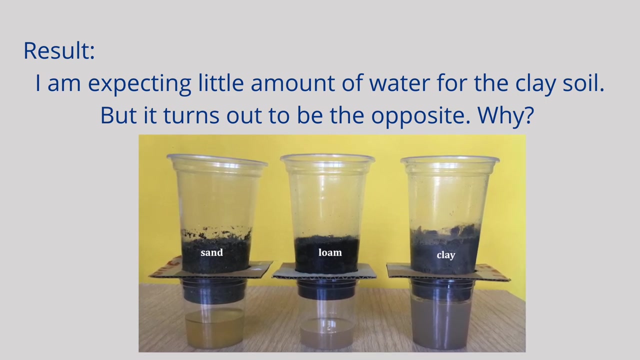 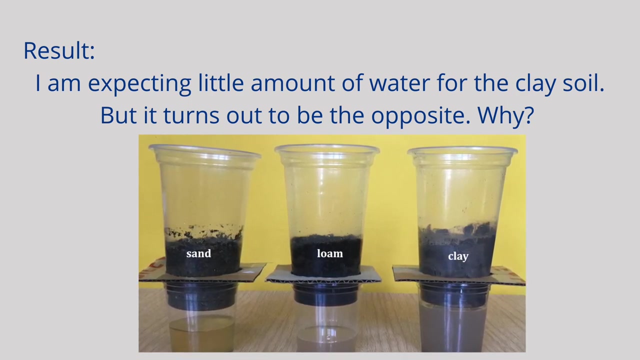 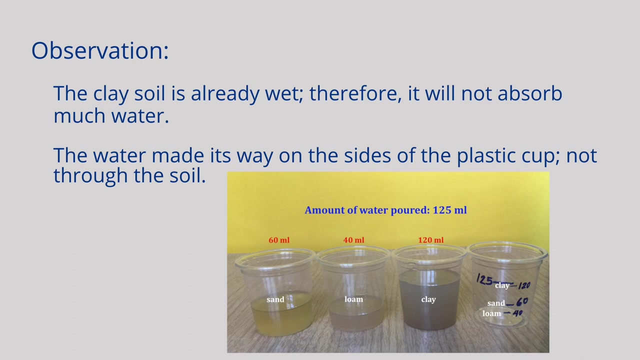 The water is measured and the timer is set, I am expecting little amount of water for the clay soil, but it turns out to be the opposite. Why, Based on my observation, the clay soil is already wet. Therefore, the water is not enough. 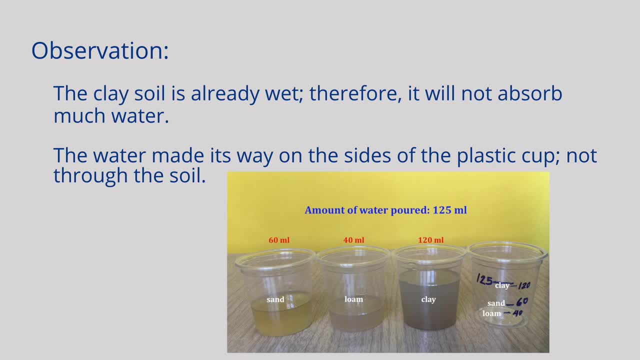 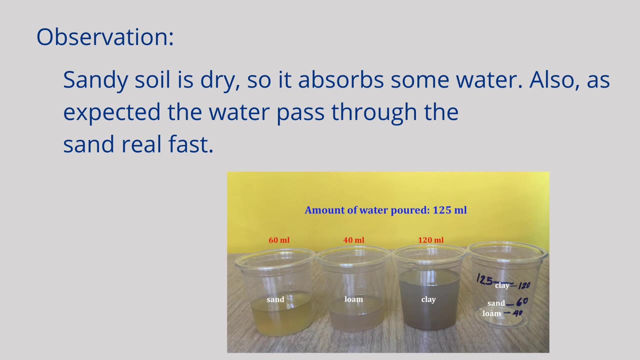 Therefore, the water is not enough. It will not absorb much water. Also, the water made its way on the sides of the plastic cup, not through the soil. On the other hand, sandy soil is dry, So it absorbs some water.